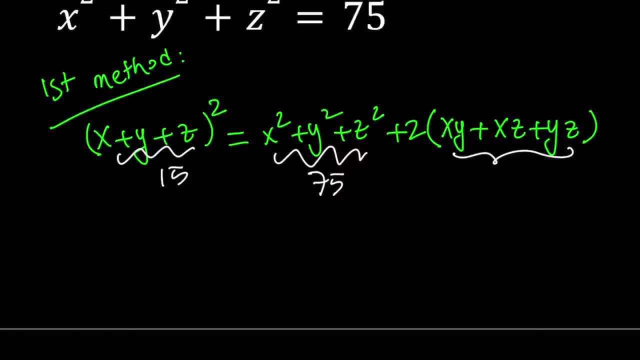 xy plus xz plus yz. So if you square 15, you get 225.. And then that is equal to 75 plus 2 times xy plus xz plus yz. If you subtract 75, you get 150.. And if you divide by 2, you get half of 150, 75.. 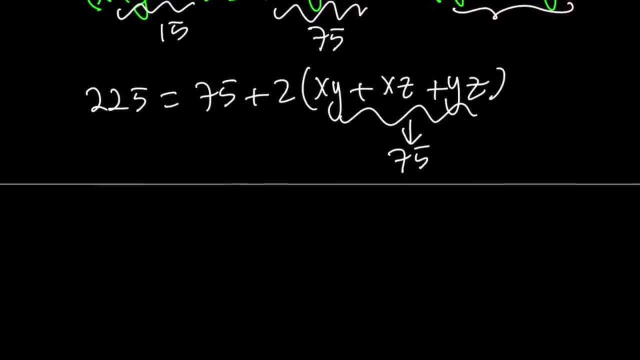 Okay, great, I mean you can do that. It's easy. It's just two steps, but I didn't show both steps, So this gives you 75.. So what? We have three equations. now Let's rewrite them. 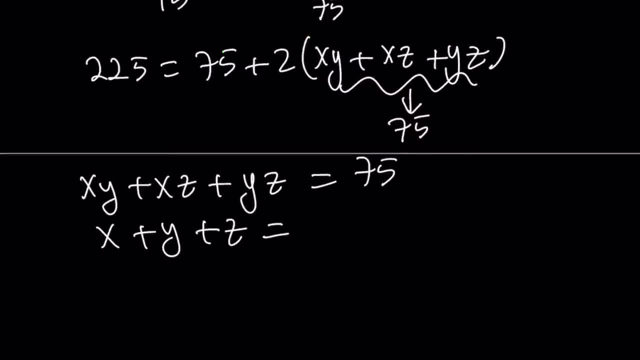 We have x plus y plus z equals 15.. We have xy, xz, yz equals 75.. We have x squared plus y squared plus z squared, equals 75.. Now you have three equations and three unknowns, so that kind of looks like a normal system. 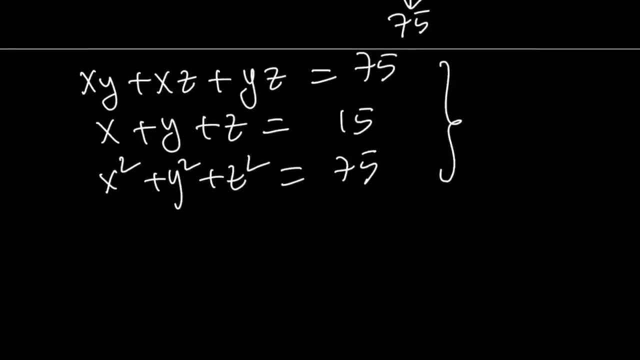 But the problem is, if you just try to solve this with the three equations, you're kind of going around in circles. So we have to do something smarter, And this is what it looks like. So this is kind of like a very special scenario. 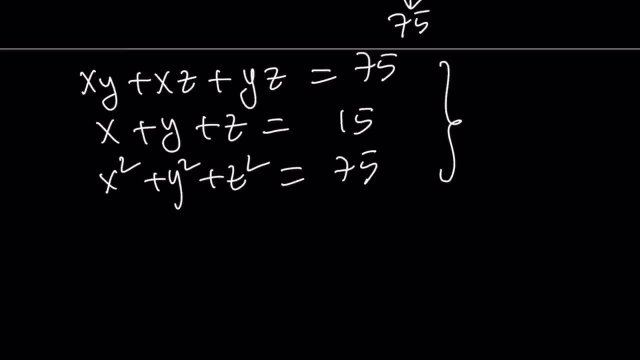 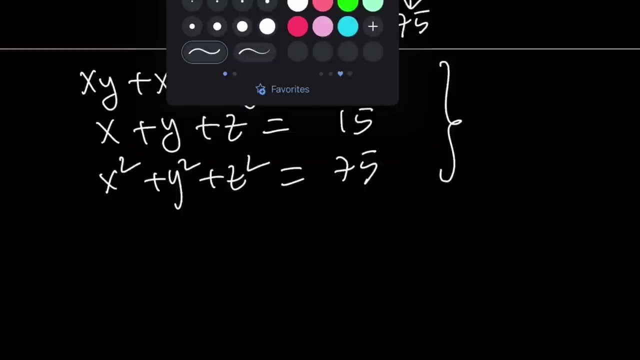 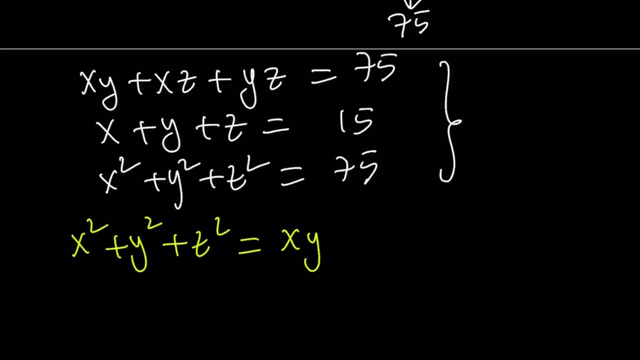 where you have the x squared plus y squared plus z squared being equal to xy plus xz plus yz. So let's go ahead and write that down as a different equation. So x squared plus y squared plus z squared is the same as xy plus xz plus yz. 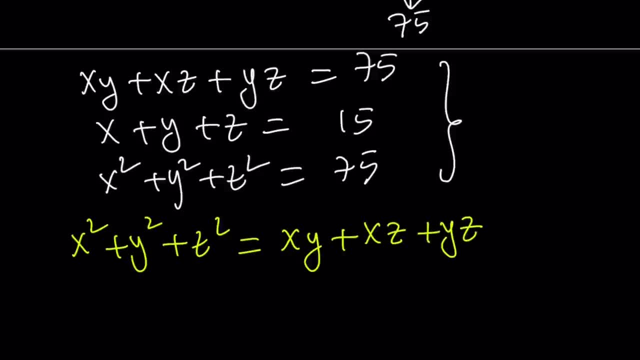 And this is significant- Why? Let me tell you why. We're going to put everything on the same side, We're going to manipulate this a little bit And then, at the end, we're going to arrive at a very interesting result. 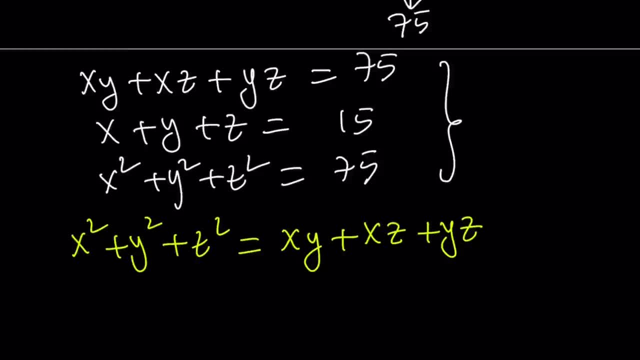 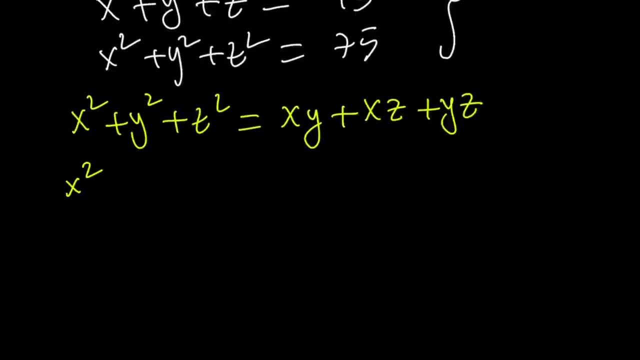 For my second method, I'm going to totally use a different approach, but before I'm also going to show you a graph. Anyways, Let's go ahead and manipulate this. We can put everything on the same side. So subtract this sum, Set it equal to zero. 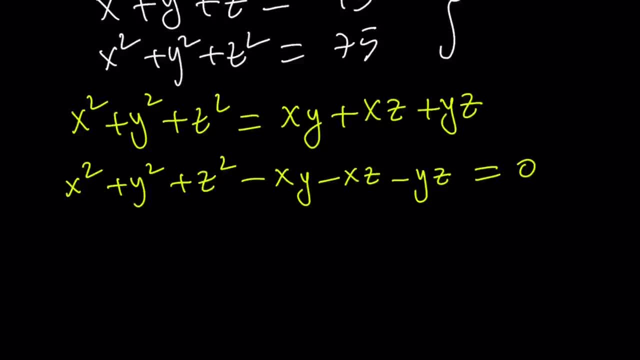 Now, in order to get some perfect squares from the left hand side, we're going to complete the squares, but we do need the right coefficients And we need a two in front of the xy, because if you have x squared minus two xy. 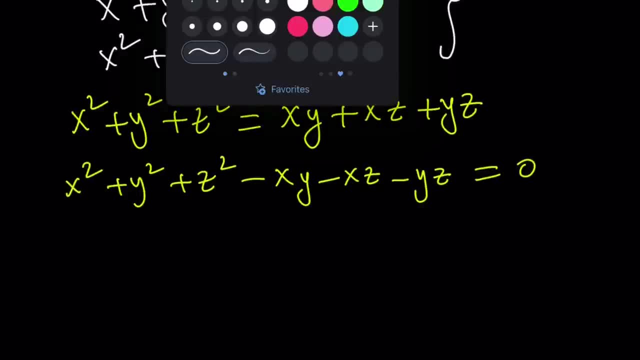 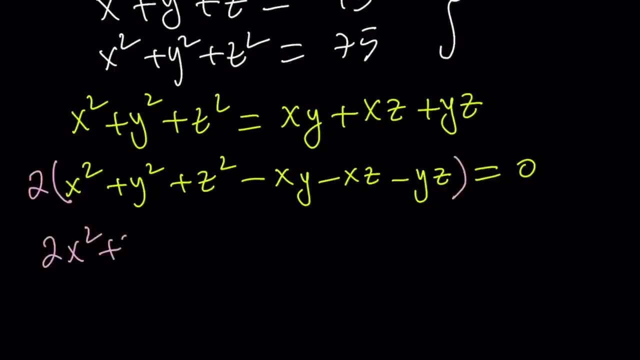 yes, we can complete the square, So let's go ahead And multiply both sides by two, which wouldn't hurt the whole thing, right, Because it's still zero. Now we get two x squared plus two y squared plus two z squared, minus two xy, minus two xz, minus two yz equals zero. 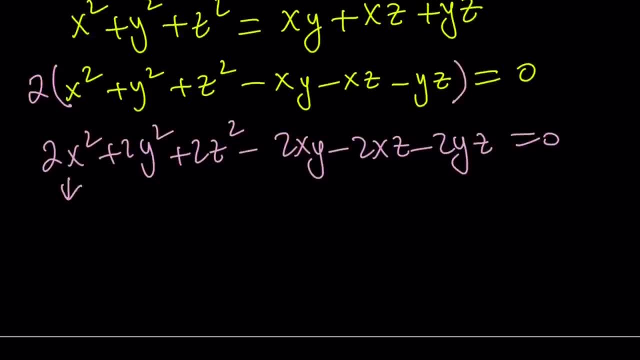 So this is nice, because now I can go ahead and break this down to x squared. I can write it as x squared and then take the negative two xy and then just attach a y squared. So I also use one of the y squared And then I can just do this with x squared again, because I have two x squared minus two xz. 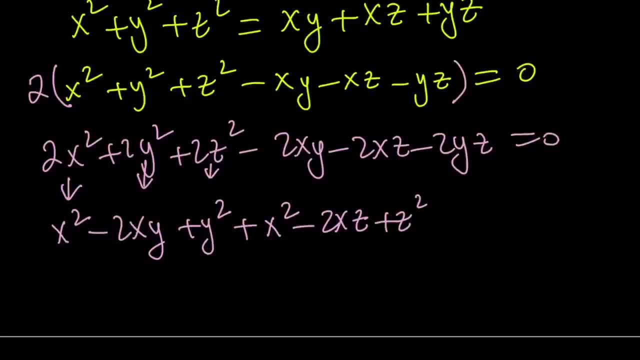 Now I want to use one of the z squared, So that's going to give me this. And now what is left? We have the y squared minus two. yz plus z squared equals zero. If you add these all up, you're going to get two x squared, which is this one. 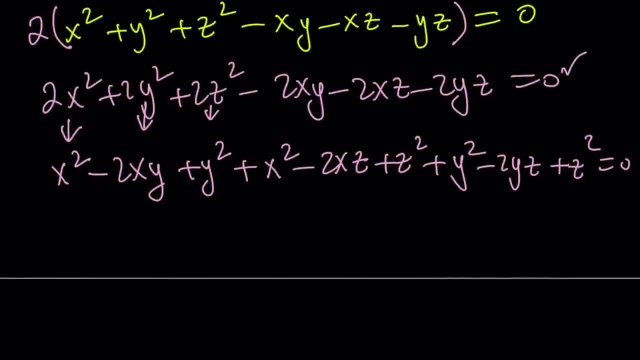 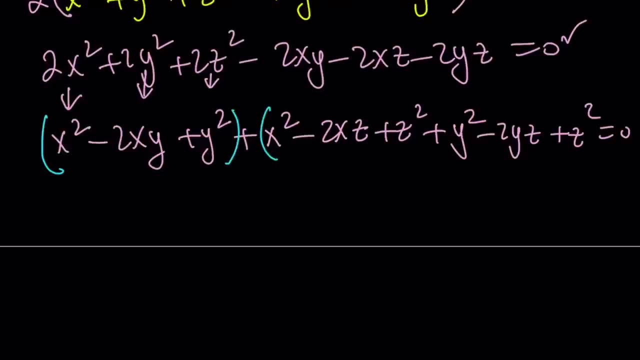 Two x squared plus two y squared, so on and so forth. So these equations are equivalent, But this second one is much, much better, because- take a look at this, This is a perfect square. This is a perfect square, And this is a perfect square. 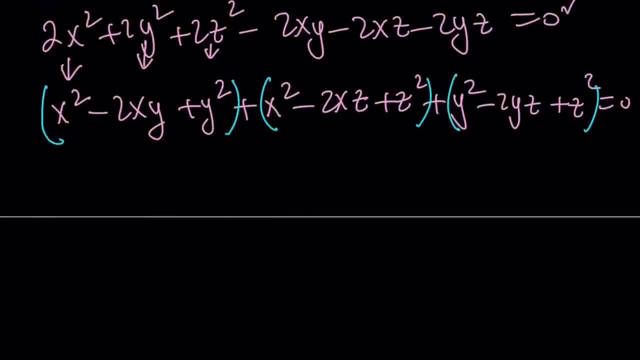 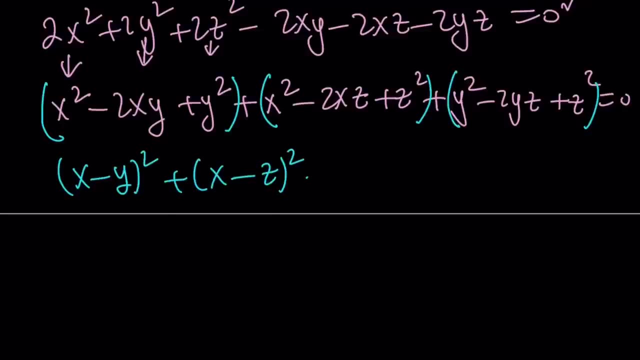 And everything is perfect, Everything is awesome, All right, So now we can write it as: x minus y- quantity squared, x minus z- quantity squared and y minus z- quantity squared, And that is equal to zero. And what does that tell you? 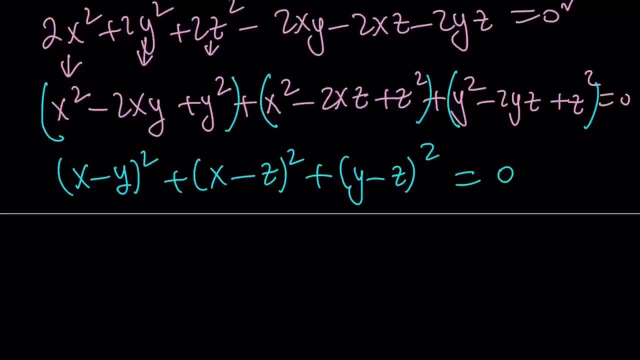 If x, y, z are real numbers- Wait a minute. Did I say they're real numbers? Well, you can also look for complex solutions, but I'm going to find the real deal. So if x, y, z are real, 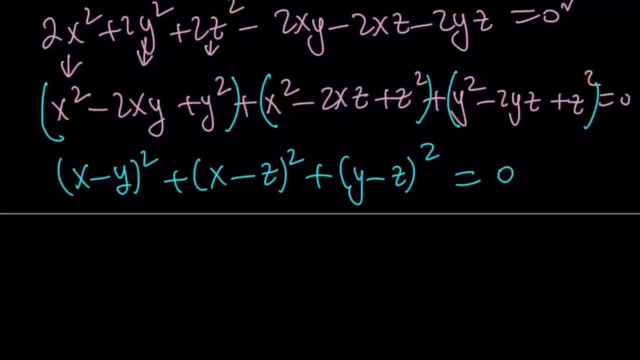 Then you can only get a sum from. you can only get a zero by adding squares. if each one is a zero, right? Because think about it, You can get a squared plus b squared is equal to zero, And either a and b are both zero or one of them has to be positive. 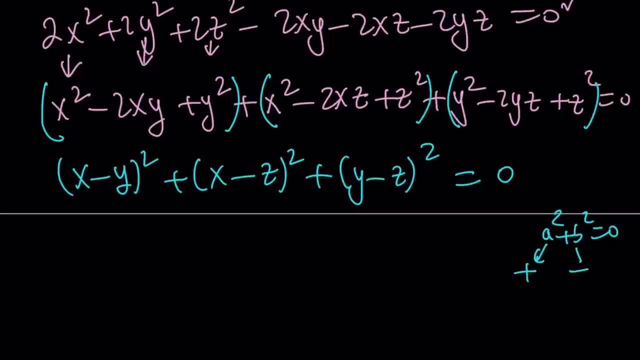 The other one has to be negative, But b squared cannot be negative in the real world. Therefore, everything has to be zero. So, and of course the three variables won't make a difference. So this has to be zero, This has to be zero. 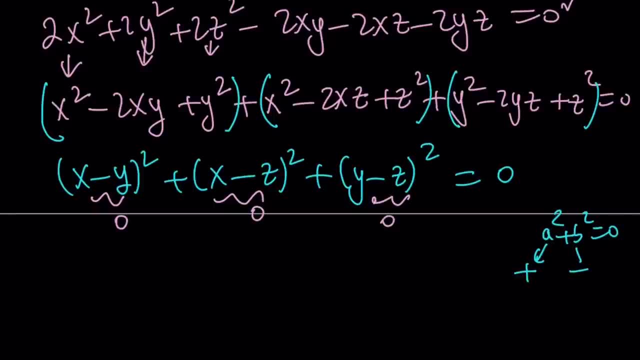 And this has to be zero, because their squares have to be zero, But it means they're zero. So from here you get the following: x equals y, y equals z, x equals z, which means x equals, y equals z, And this is a very important result, because this is where we come from. 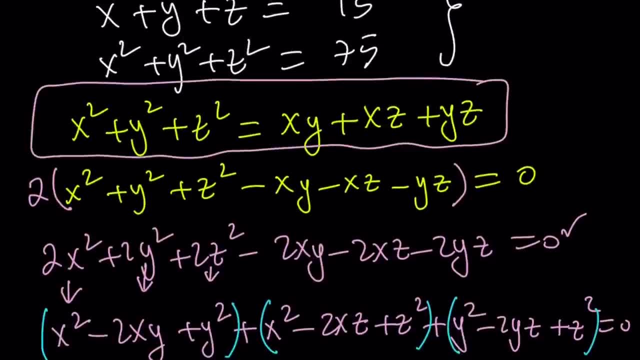 Remember that right. So whenever you have this equality, that means x, y, z are all equal. Think about it: If x and y are equal, x y becomes x squared or y squared or z squared, right, So that's a really cool result. 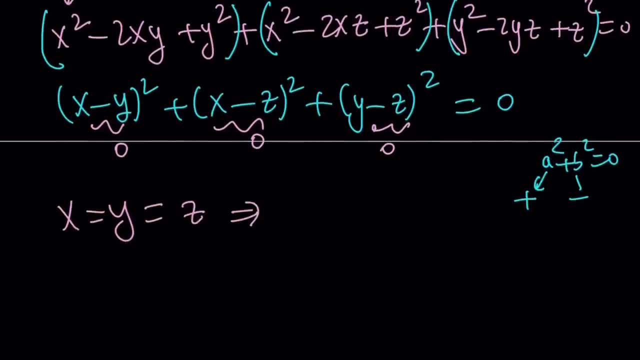 If they're all equal, then we know that their sum is 15.. So each number is going to be 5,, 5, and 5.. And that is the end of the first method. Now let's go ahead and talk about the second method. 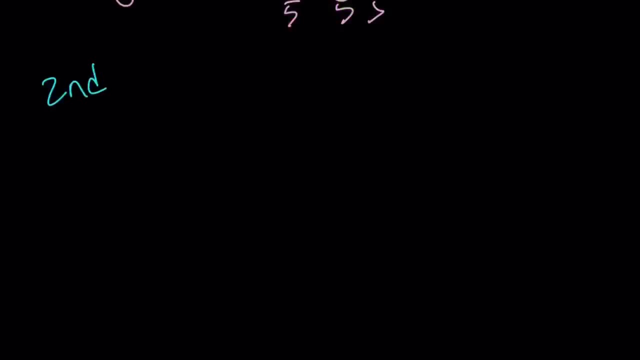 The second method is kind of different, And for the second method I'm going to show you a graph, But before that, let's go ahead and manipulate this. Okay, We have: x plus y plus z is equal to 15.. From here, I would like to know: 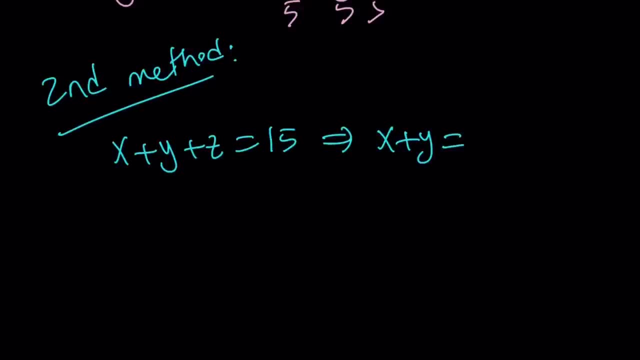 I have to isolate z or x plus y. rather, I can write x plus y as 15 minus z, And I know that their sum, the squares of their sum, is 75.. So from here I can isolate x squared plus y squared and write it as 75 minus z squared. 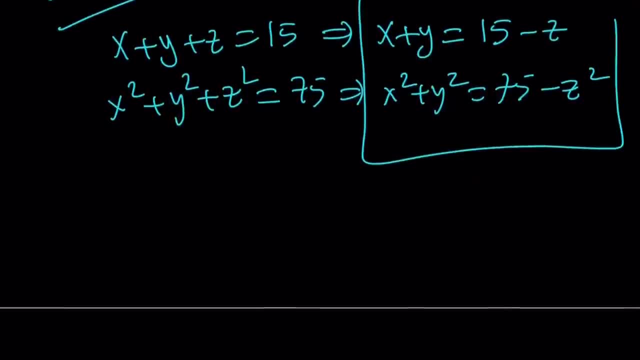 Great. What does that give you? A system of equations in two variables. Forget about the z. Z is a parameter. We're just going to play with it. Now remember the identity, which is x plus y squared equals x squared plus y squared plus z squared. 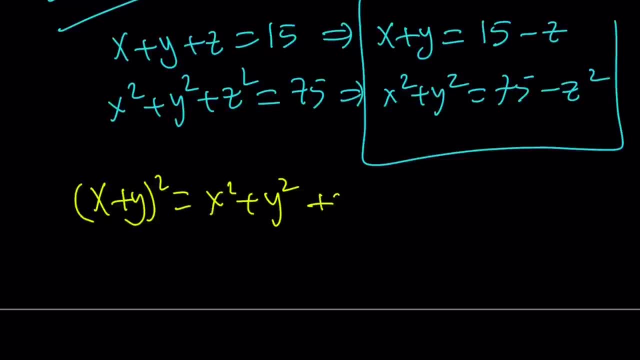 Oops, there's no z, Never mind Plus 2xy. Get carried away Now. x plus y is 15 minus z, So we're going to square that. x squared plus y squared can be written as 75 minus z squared plus 2xy. 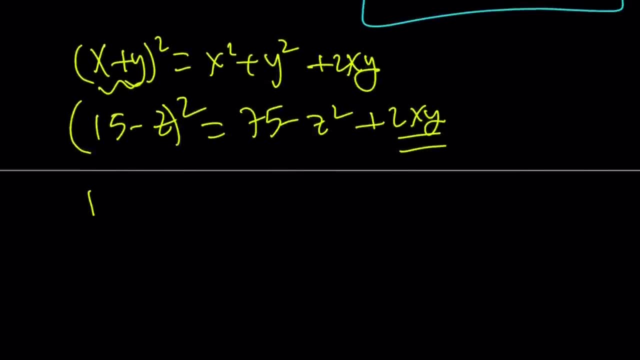 Now, from here we can solve for xy Right: 15 minus z squared is 225 minus 30z plus z squared, And then you can just go ahead and bring these, Bring these over And then isolate the 2xy. 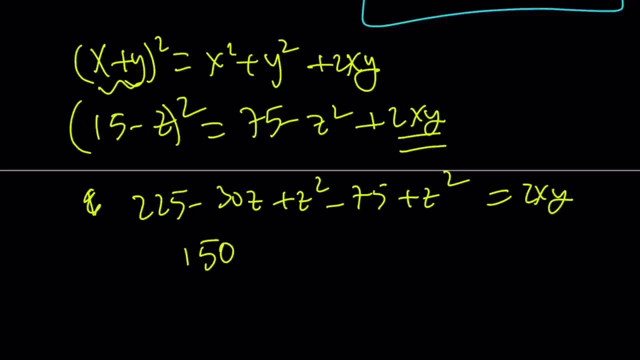 And if you simplify this a little bit, you're going to get 150 minus 30z plus 2z squared. Let's go ahead and write down 2z squared first, And maybe I'm just going to follow it up with the 30z so we can write it in the standard form. 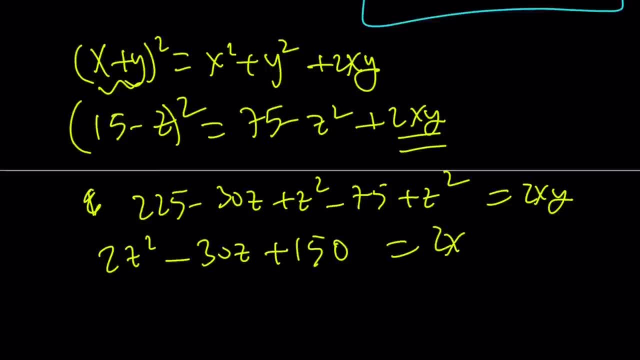 Right Plus 150. This is equal to 2xy. If you divide both sides by 2, you're going to get xy, which can be written as z squared minus 15z plus 75.. Now we're going to use Viettas formulas. 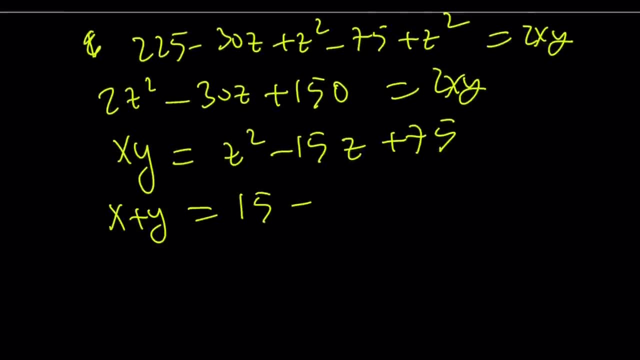 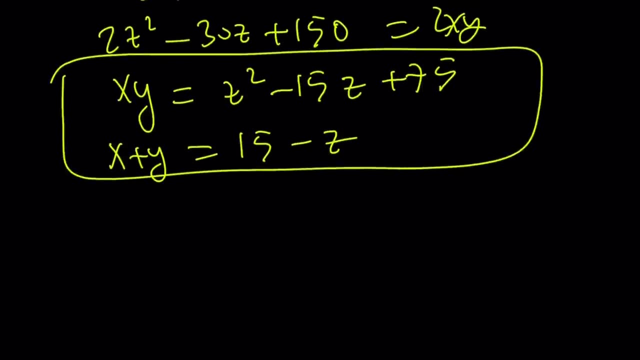 Why? Because we know xy and we know x plus y, So we can kind of write the equation whose roots are x and y. Let's use a different variable like t. Right, I like t, by the way. I don't know if you like it. 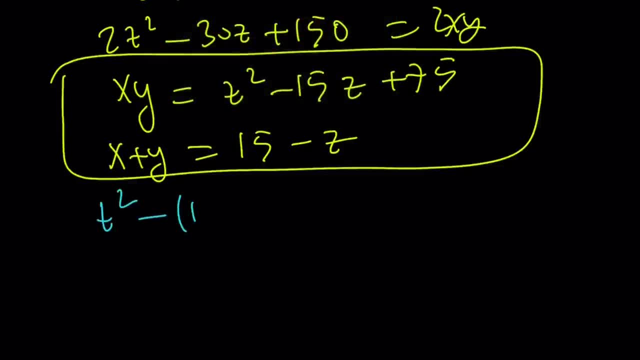 If you like it, comment down below: t squared minus 15 minus z, t plus z squared minus 15z plus 75.. This is an equation whose roots are x and y, But notice that this is the opposite of the sum that comes in here. 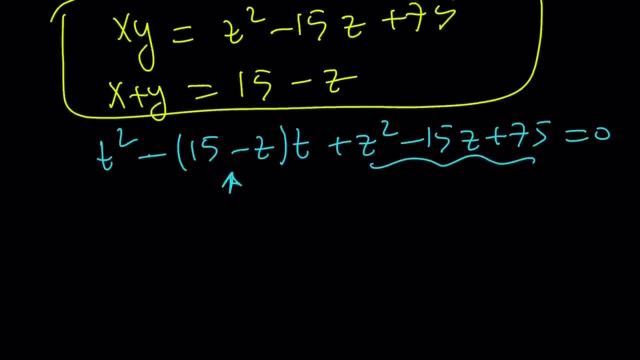 And this is the product from Viettas formulas. Right, And what am I going to look at? I'm going to find the discriminant b squared minus 4ac, And this is going to give you something very interesting. Take a look. 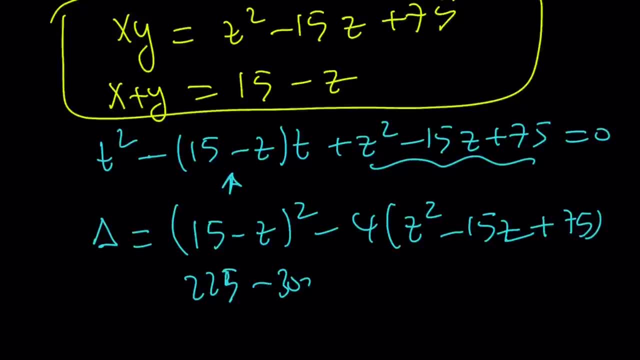 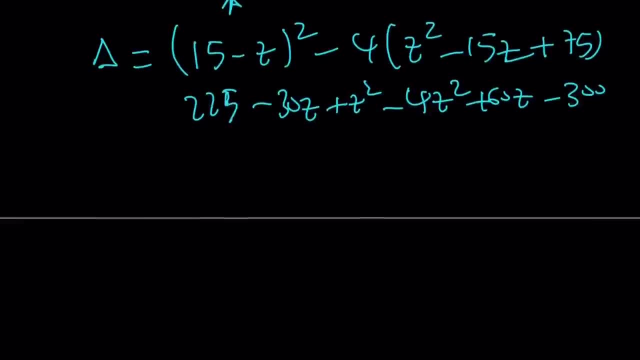 This is 225 minus 30z, plus z squared, minus 4z squared, plus 60z minus 300.. Okay, This is going to give you z squared minus 3.. 4z squared is going to give you negative 3z squared. 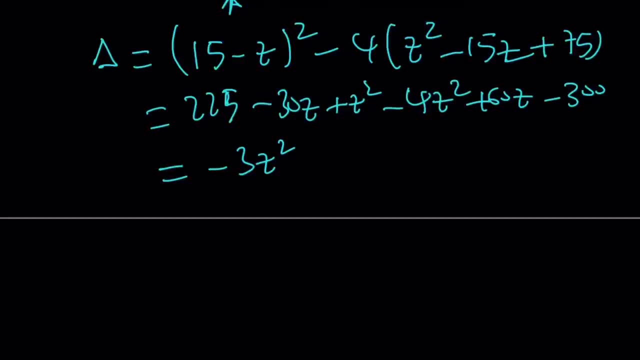 And then you're going to get negative 30 plus 60z, That's going to be positive 30z. And then, finally, you have the 225 minus 300, which is negative 75. And guess what? You can take out a 3.. 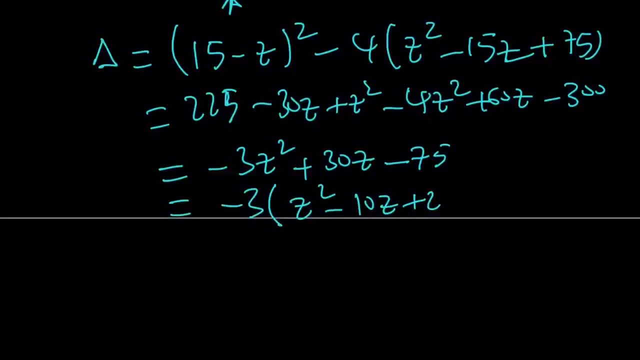 Negative 3, I mean z squared minus 10z plus 25. And this becomes equivalent to z minus 5, quantity squared. This is obviously always less than 3.. Less than or equal to 0. And it can't be happening because we're looking for real solutions.